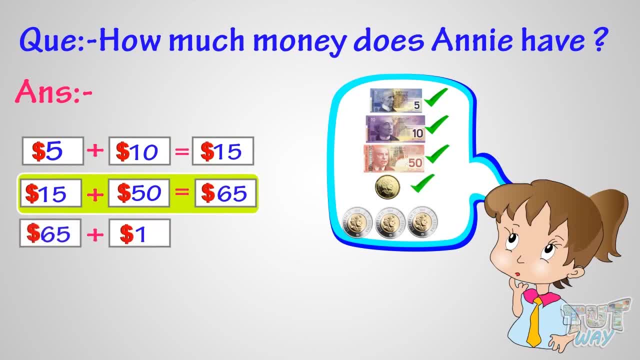 Sixty-five plus one, we get sixty-six. Sixty-six plus six, that is three toonies, we get seventy-two. So Annie has seventy-two dollars in all. Now let's move to another question, Another question. 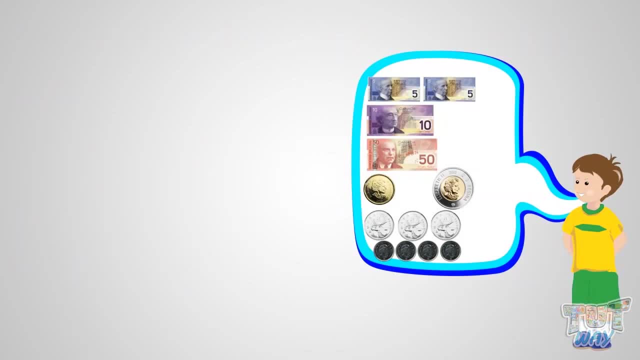 Now, if this money belongs to Sam, then how much money does Sam have? Sam has two five dollar bills, a ten dollar bill, a fifty dollar bill, a loonie, a toonie, three quarters and four dimes. 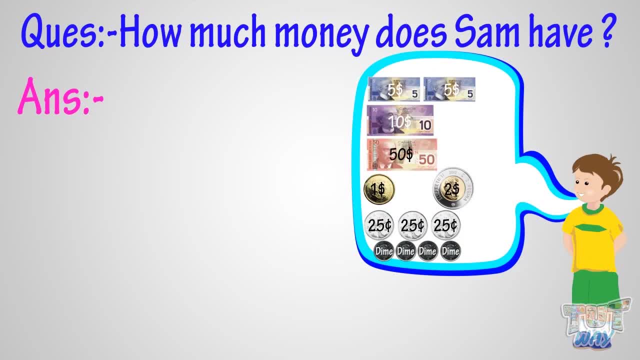 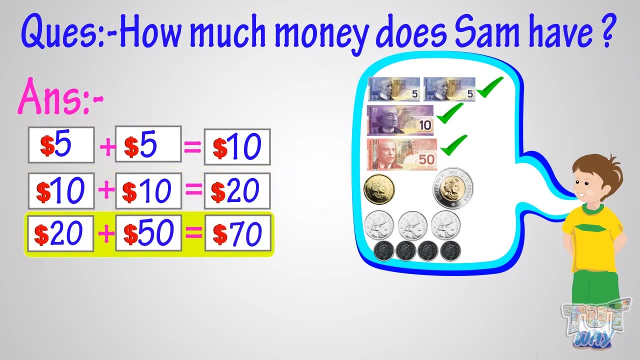 Now let's add up all to get how much money Sam has. the joyous Two five dollar bills equal ten dollars. Ten dollars plus ten dollars means twenty dollars. Twenty dollars plus fifty dollar bill equals seventy dollars. Seventy dollars plus a loonie equals seventy-one dollars. 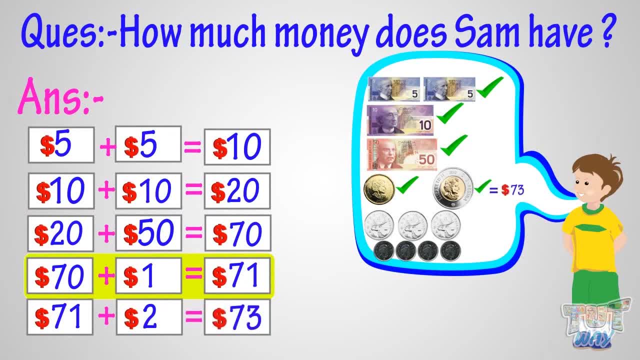 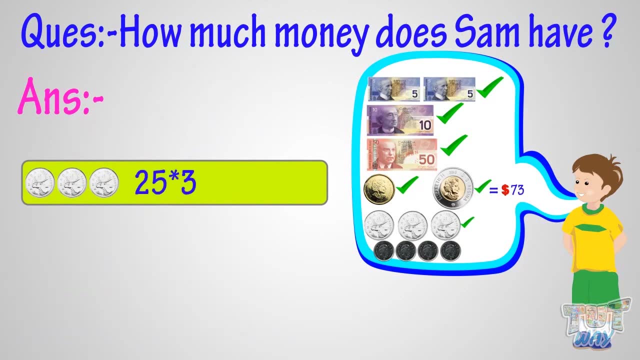 Seventy-one dollars plus a teahouse means twenty dollars. peace party是你的 longing with her Tuni equals $73.. Then we have 3 quarters and 4 dimes. 3 quarters equals 25. multiplied by 3 equals 75 cents. $73 plus 75 cents equals $73 and 75 cents. Now we also have 4 dimes. 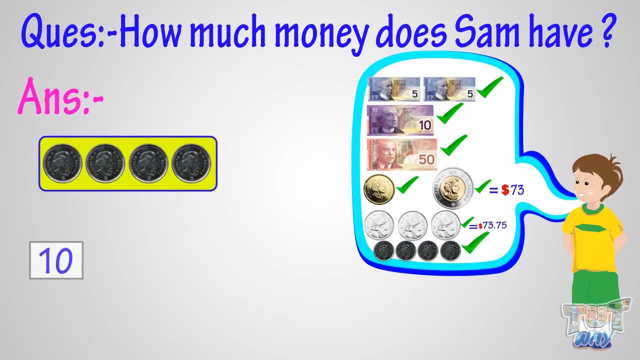 where 1 dime is 10 cents, Where 4 dimes make 40 cents. Adding 40 cents to $73 and 75 cents, we get $74 and 15 cents. So Sam has $74 and 15 cents in all. 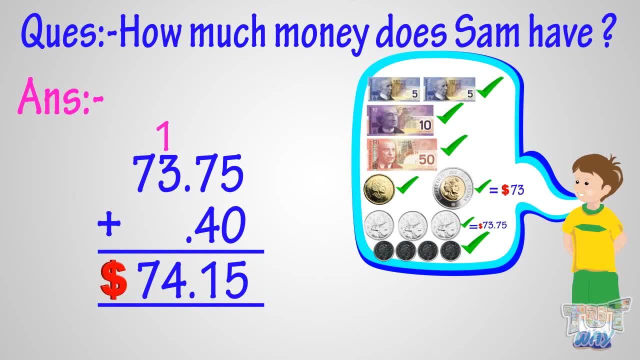 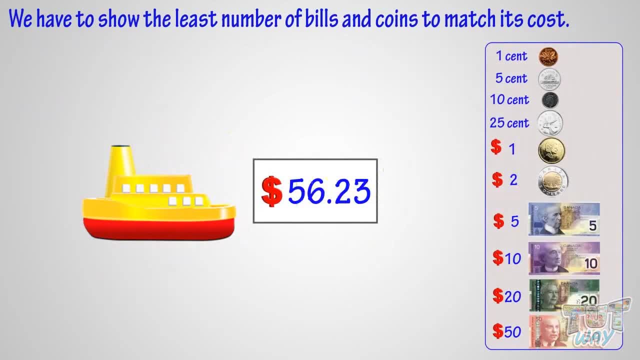 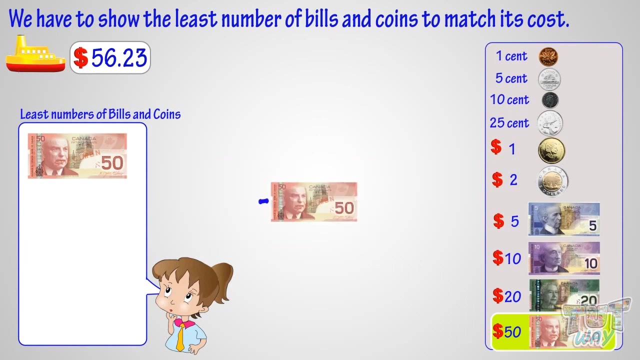 Now let's move to another question. Here is a toy with its cost mentioned. We have to show the least number of bills and coins to match its cost. $50 bill is closest to our figure of 56.23.. So take out 1 $50 bill. Now subtract $50 from. 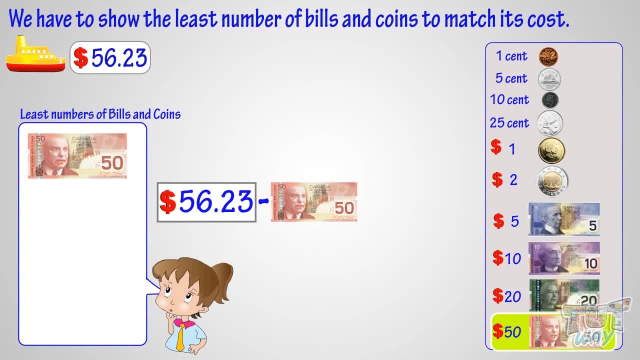 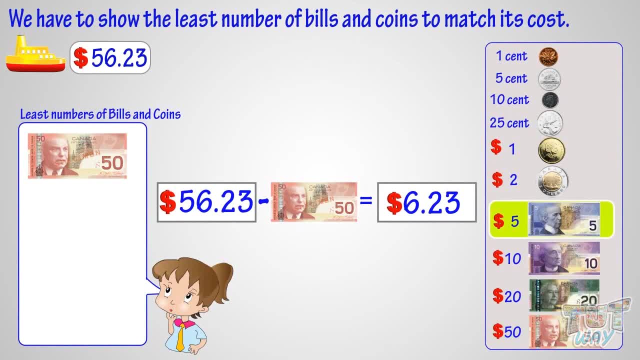 to pay. now $5 bill is closest to our figure of $6.23.. So take out one bill of $5.. Now subtract $5 from $6.23.. Now we are left with $1.23.. So next we can take out one bill of. 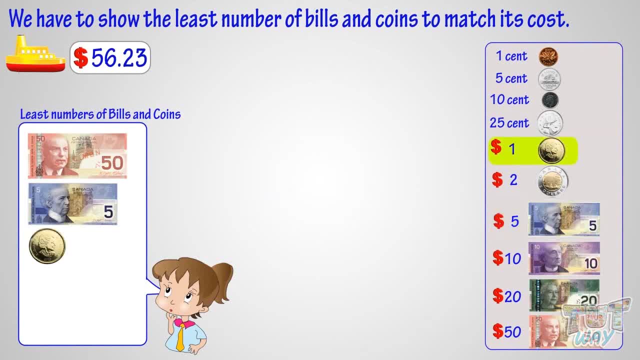 $1 coin. That's a loonie. Now subtract $1 from $1.23.. And we are left with $0.23.. This amount is less than a quarter, So we will use two dimes to make $0.20.. Now we are left. 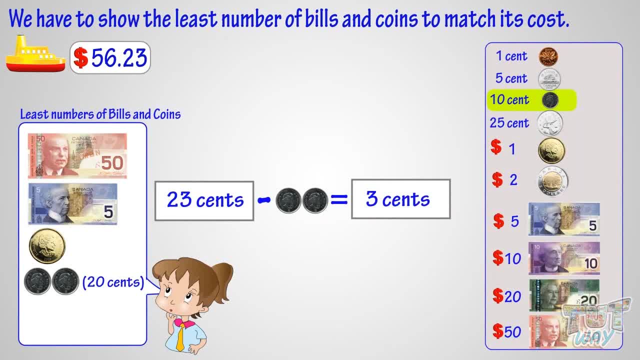 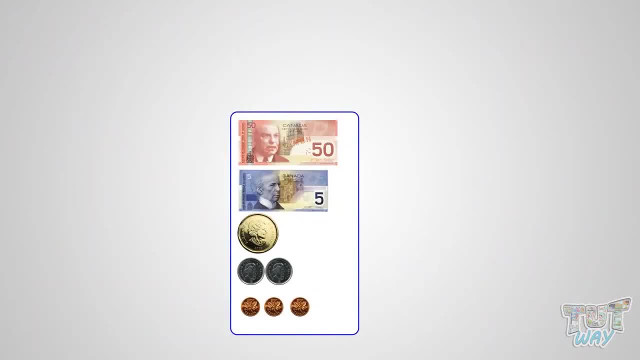 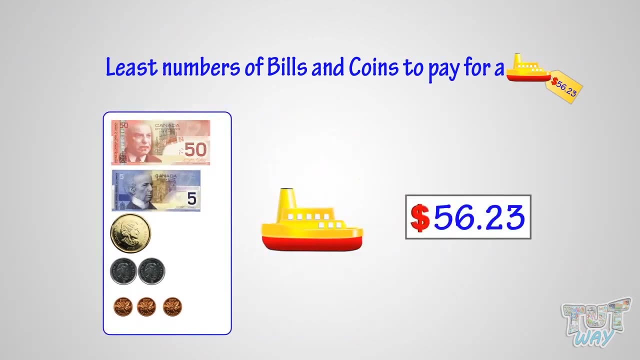 with only $0.03.. So we can use three pennies. Yes, we are done. We have selected bills and coins to pay for a toy of $56.23.. Now let's take another example. Here is a toy car with its cost mentioned. 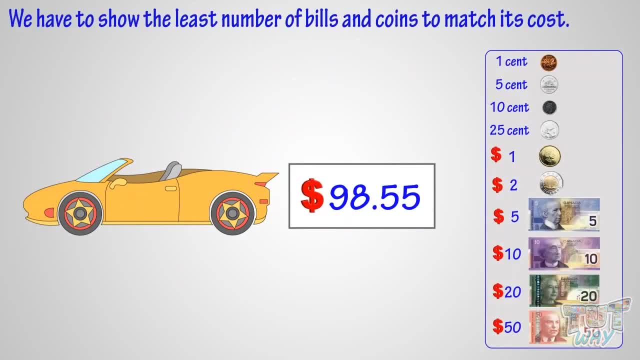 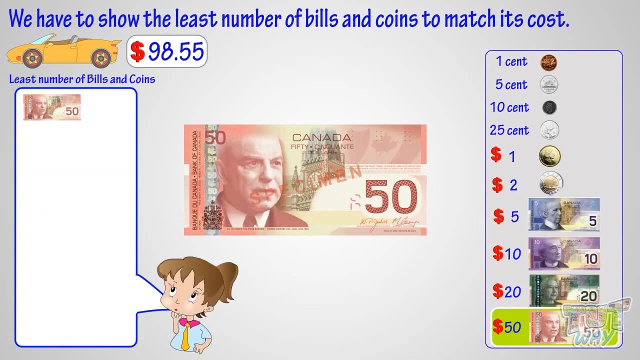 We have a toy car with its cost mentioned. We have a toy car with its cost mentioned. We have to show the lease bills and coins to match its cost. The amount is more than the biggest bill we have, That is $50.. So take out one $50 bill Now, subtract $50 from $98.55.. Now we are left. 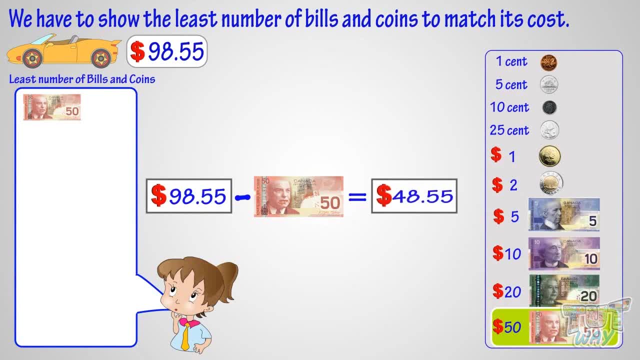 with $48.25.. Now subtract $48.55.. This amount is less than a $50 bill. So next biggest bill we have is $20 bill. So take out one $20 bill. Now subtract $20 bill from $48.55.. 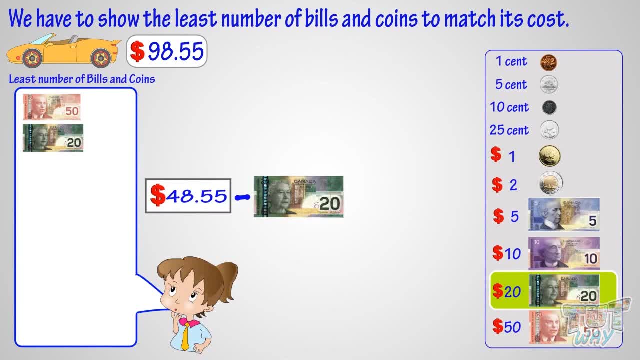 Now we are left with $28.55.. Again, this amount is bigger than a $20 bill. So take out one $20 bill Now, subtract $20 bill from $28.55.. And we are left with $8.55.. 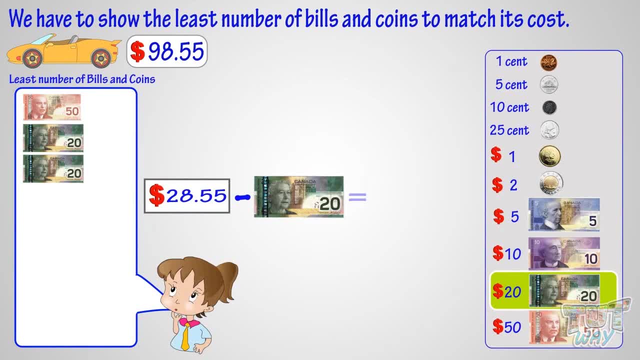 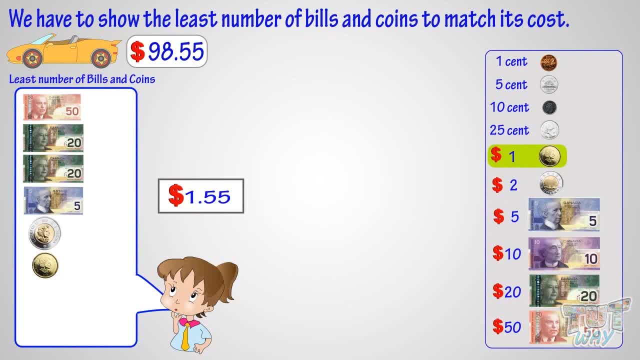 Now subtract $20 bill from $28.55. And we are left with $28.55.. Now subtract $20 bill from $28.55. And we are left with $28.55.. A dollar and fifty-five cents minus one dollar equals fifty-five cents. 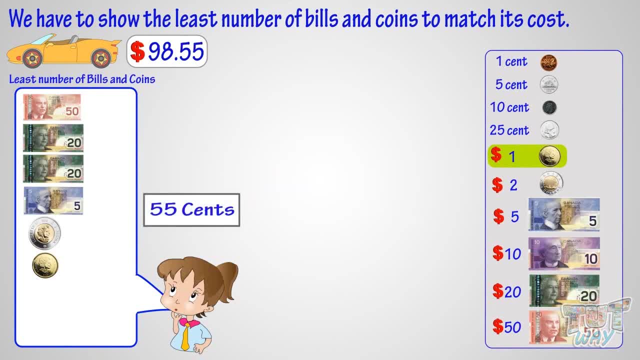 Now we are left with fifty-five cents. amount is less than a dollar, So we will have to use smaller coins than a Looney. So we will use a quarter And subtract Twelve 25 cents from 55 cents, So we will be left with 30 cents to pay now. 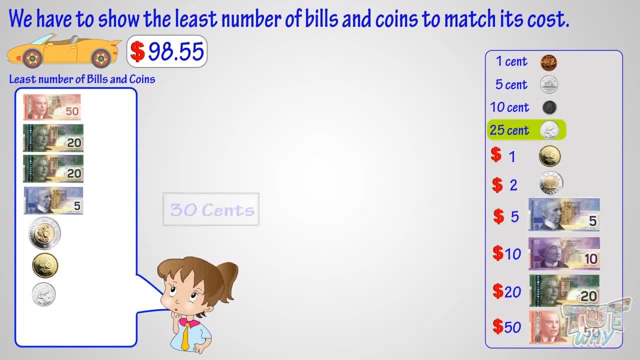 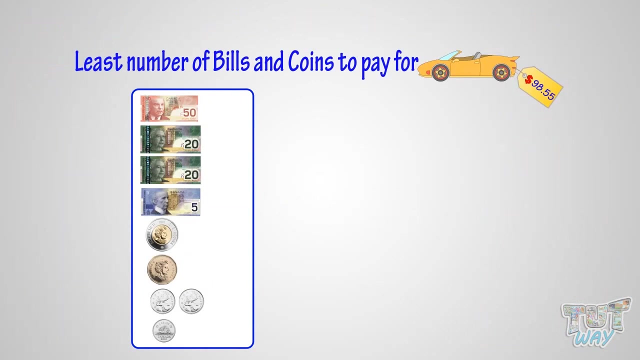 So again, we can take out a quarter and subtract 25 cents from 30 cents And we are left with 5 cents to pay now, And for that we can use a nickel. Yes, we are done. We have selected the least number of bills and coins to pay for a toy of $98.55. 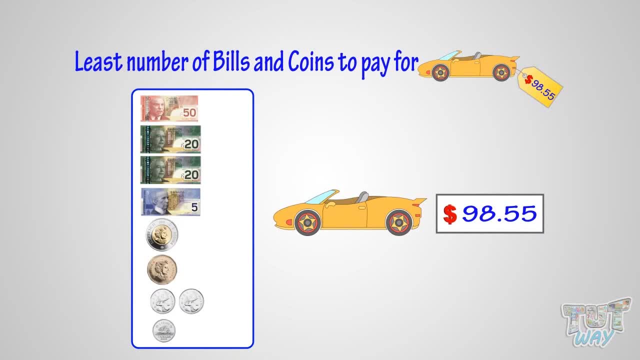 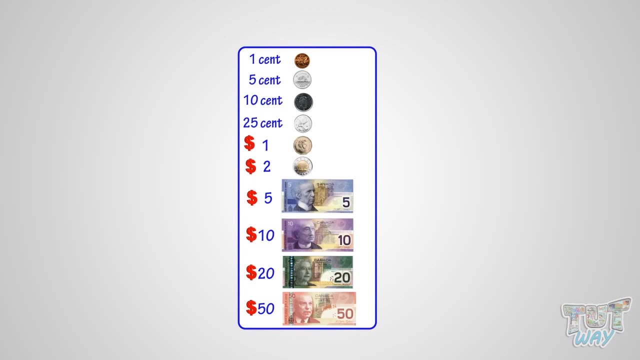 Least number of bills and coins to pay for this toy can be this. So, kids, today we learned making money amounts up to $100. And using the least number of bills and coins for that. Now you can go shopping with your mom and use your savings. 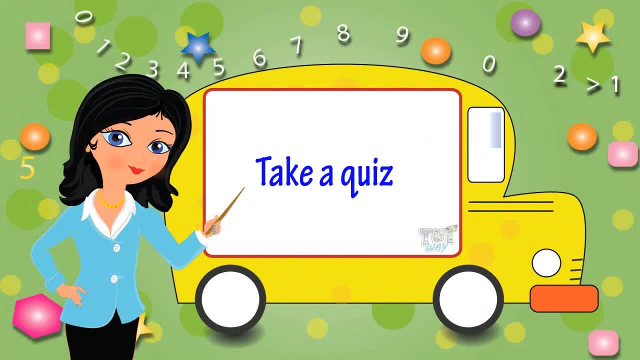 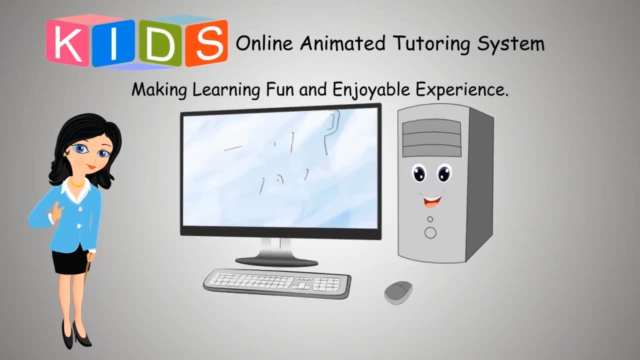 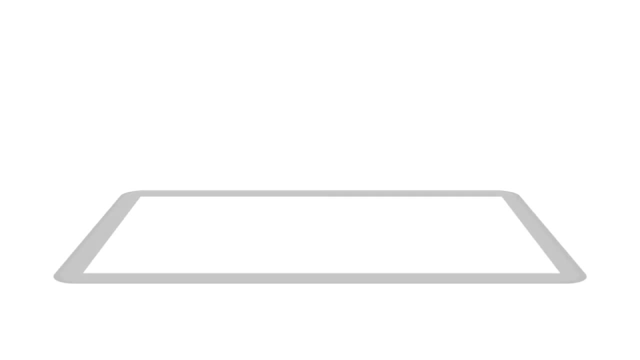 Bye-bye, Bye-bye, Bye-bye, Bye-bye, Bye-bye, Bye-bye.